So we're asked to graph: f of x is equal to two times the absolute value of x plus three plus two. And what they've already graphed for us, this right over here, this is the graph of y- is equal to the absolute value of x. 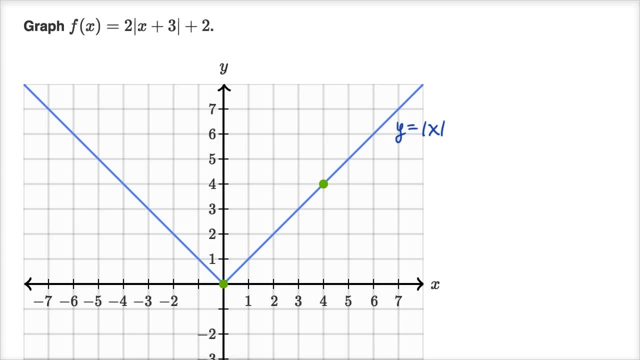 So let's do this through a series of transformations. So the next thing I wanna graph- let's see if we can graph y: y is equal to the absolute value of x plus three. Now, in previous videos we have talked about it. 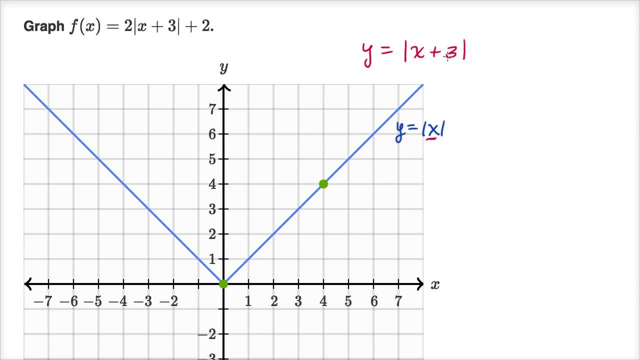 If you replace your x with an x plus three, this is going to shift your graph to the left by three. You could view this as the same thing, as y is equal to the absolute value of x minus negative three, And whatever you are subtracting from this x. 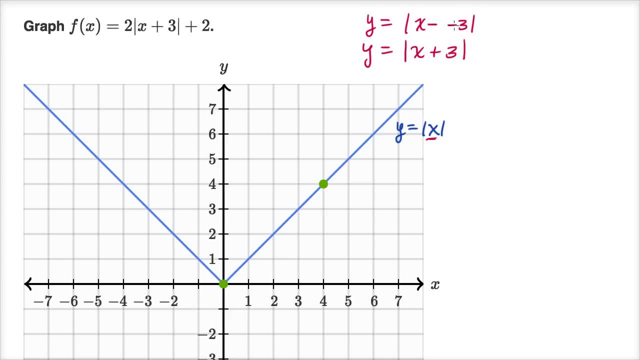 that is how much you are shifting it. So you're going to shift it three to the left And we're gonna do that right now and then we're just gonna confirm that it matches up, that it makes sense. So let's first graph that and get my ruler tool here. 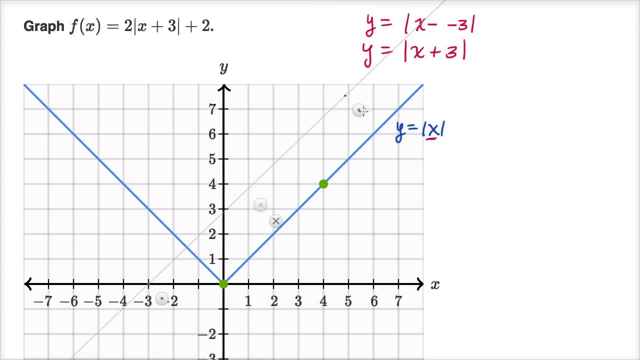 So if we shift three to the left, it's gonna look something like, it's gonna look something like this. So, on that, when whatever we have inside the absolute value sign is positive, we're going to get essentially this slope of one. 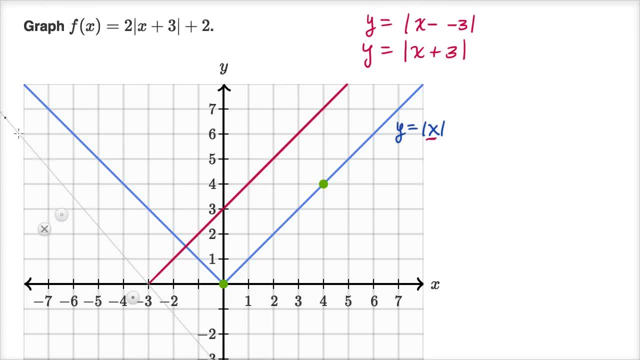 And whenever we have inside the absolute value sign is negative, we're gonna have a slope of essentially negative one. So it's gonna look. it's going to look like that And let's confirm whether this actually makes sense. Below x equals negative three. 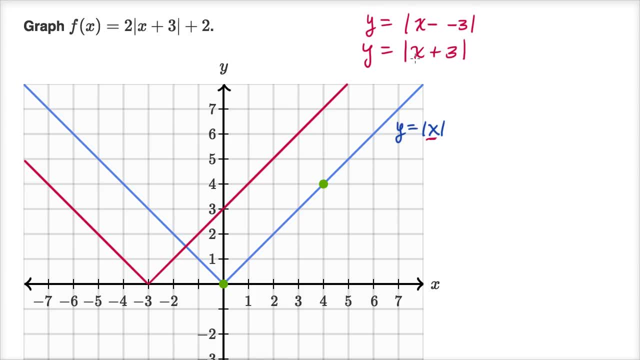 for x values less than negative three. what we're gonna have here is this: inside of the absolute value sign is going to be negative, and so then we're gonna take its opposite value, and so that makes sense. That's why you have this downward line right over here. 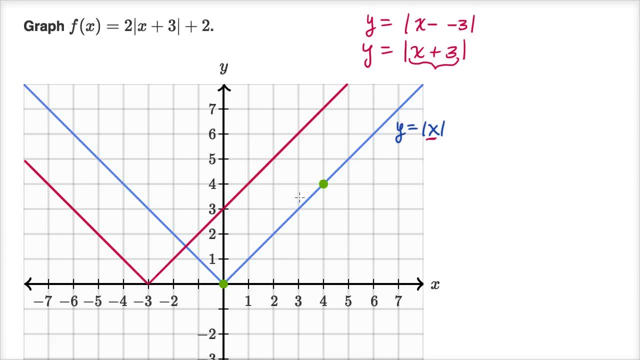 Now for x's greater than negative three. when you add three to it, you're going to get a positive value, and so that's why you have this upward sloping line right over here. And at x equals negative three, you have zero inside the absolute value sign. 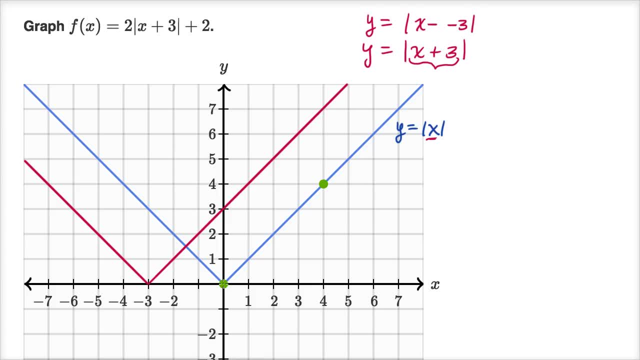 just as if you didn't shift it, you would have had zero inside the absolute value sign at x equals zero. So hopefully that makes a little bit more intuitive sense of why if you replace x, if you replace x with x, with x plus three- and this isn't just true. 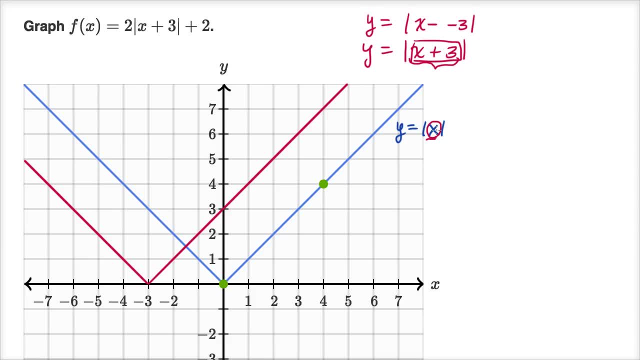 of absolute value functions. this is true of any function. If you replace x with x plus three, you're going to shift three to the left. All right, now let's keep building. Now let's see if we can graph. y is equal to two. 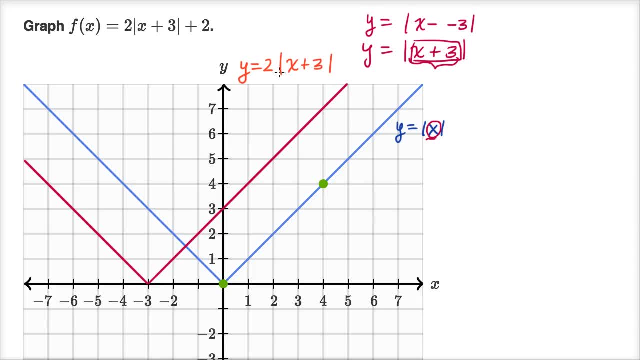 times the absolute value of x plus three. So what this is essentially going to do is multiply the slopes by a factor of two. It's going to stretch it vertically by a factor of two. So for x values greater than negative three, instead of having a slope of one. 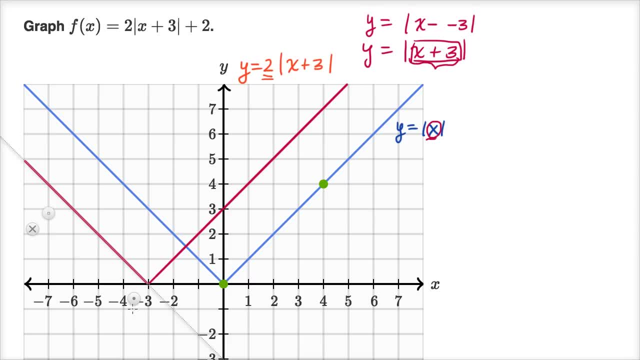 you're going to have a slope of two. So let me get my ruler out again and see if I can draw that. So let me put that there And then. so here, instead of a slope of one, I'm going to have a slope of two. 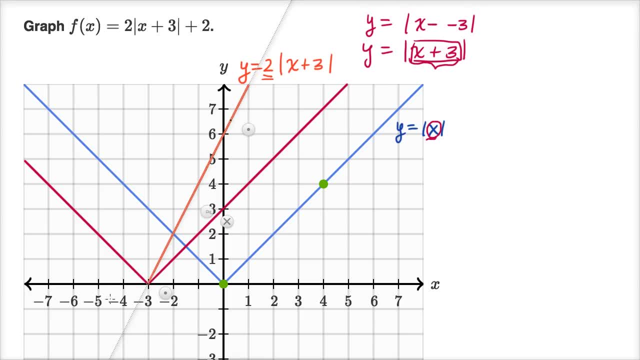 Let me draw that. It's going to look like that right over there, And then, instead of having a slope of negative one- for values less than x equals negative three- I'm going to have a slope of negative two. Let me draw that right over there. 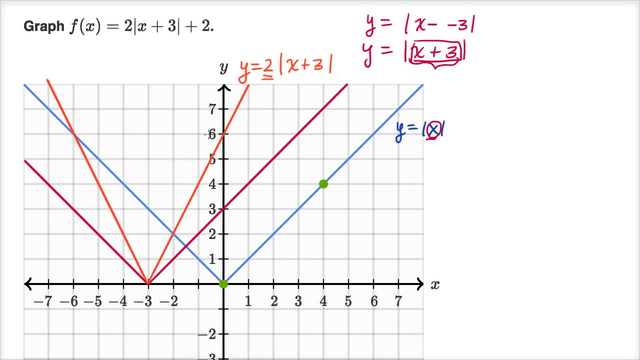 So that is the graph of y is equal to two times the absolute value of x plus three. And now to get to the f of x that we care about, we now need to add this two. So now I want a graph, and we're in the home stretch. 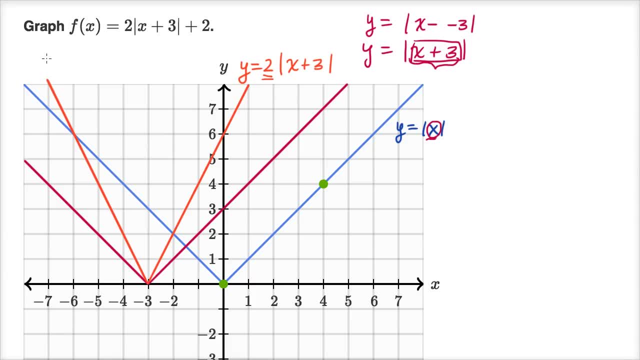 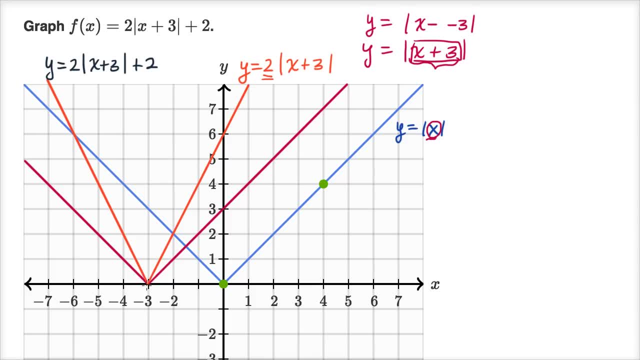 Well, whatever y value I was getting for this orange function, I now want to add two to it. So this is just going to shift it up vertically by two. So, instead of so, this is going to be shifted up by two. this is going to be shifted.